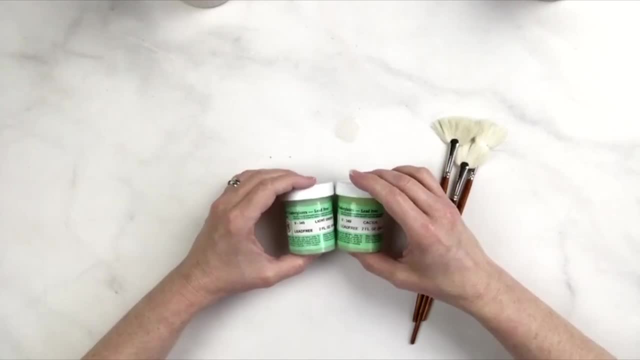 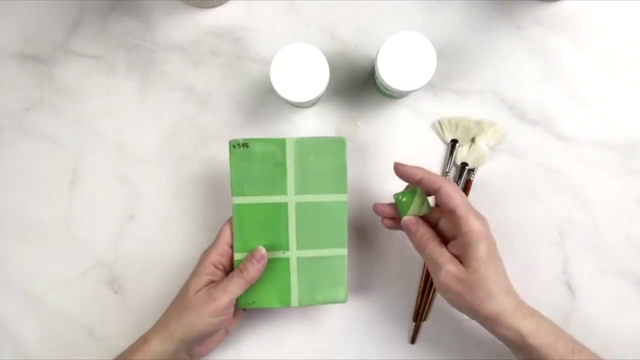 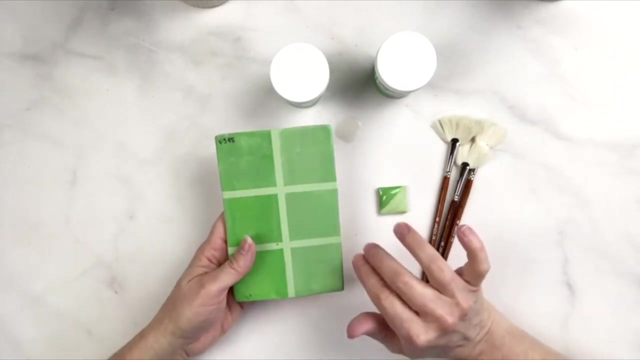 And how V345 Light Green is affected by. So these are tiles that show This is Cactus with LG10.. This is at cone 05.. So low fire. This is not with HF9 or HF10.. These are low fire glazes. 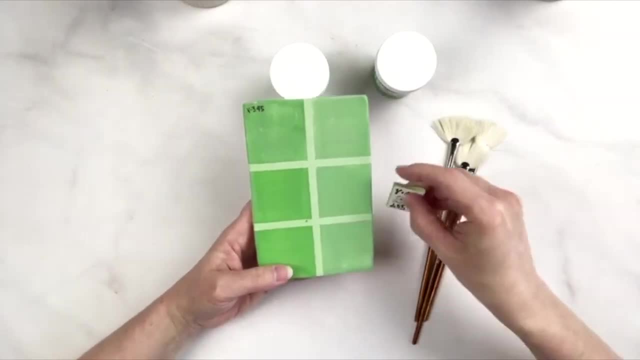 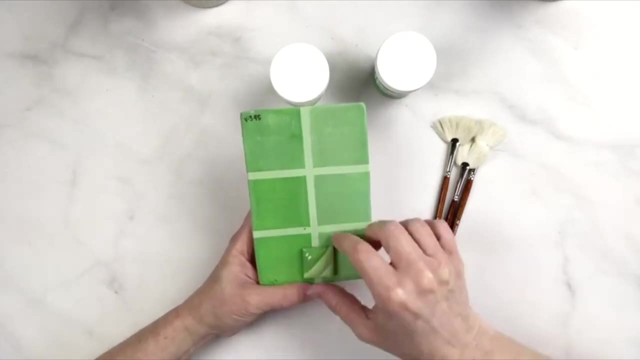 So this is 345 with LG10.. And this is 349.. So Light Green and Cactus with the same glaze And, as you can see, they look pretty much alike. There's not a lot of variation. So if you're using low fire and you're using LG10 at low fire temperatures, 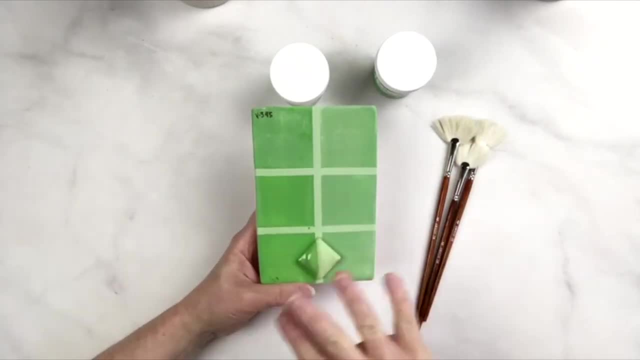 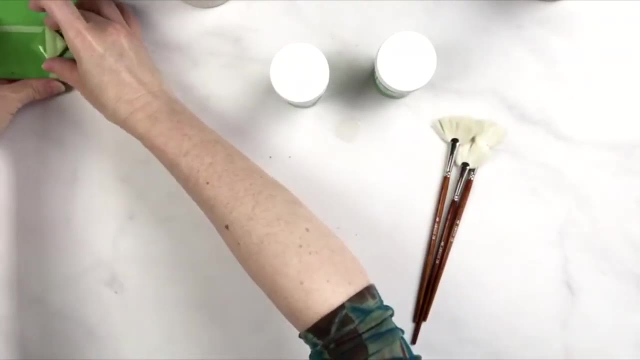 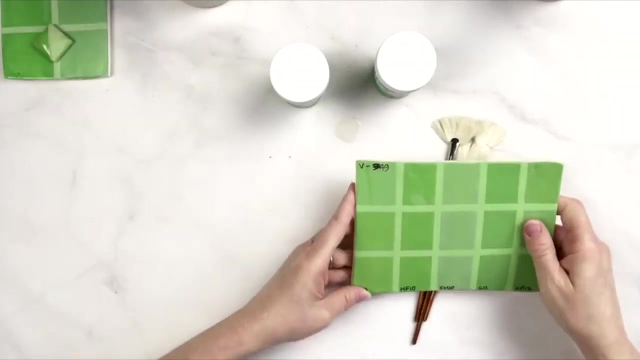 it doesn't make any difference. You can use whichever one you prefer. You're going to get a similar kind of response. Where the change comes in is when you go up to cone 05.. So this is Cactus with HF9, Zinc Free Clear. 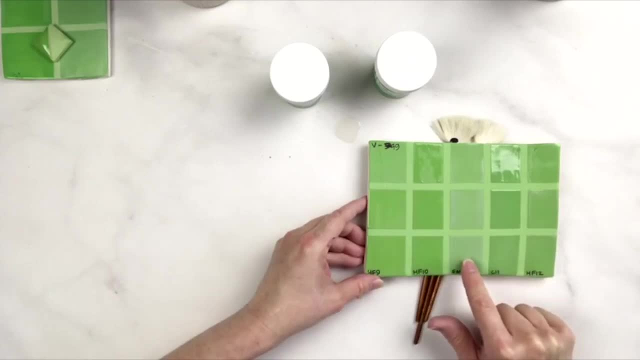 HF10, the Zinc Bearing Clear, SM10, C11, Mixing Clear And HF12.. And you can see the color is pretty much the same all the way across. There's not a lot of variation. In fact, there's almost no difference between HF9 and HF10.. 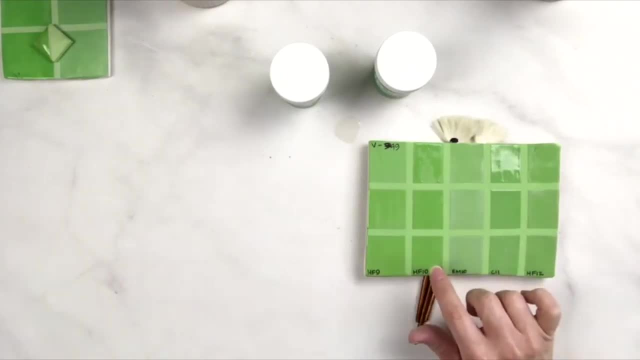 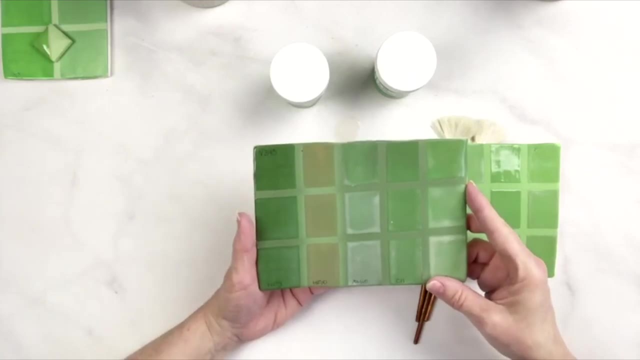 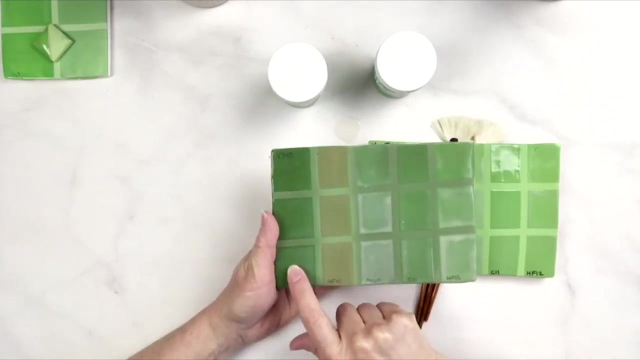 Very, very similar. That's Cactus. That's our newer under glaze. However, you can see a big difference when you switch to the V345 Light Green. This is HF10. Zinc Free Clear. This is HF9.. HF10, which has Zinc. 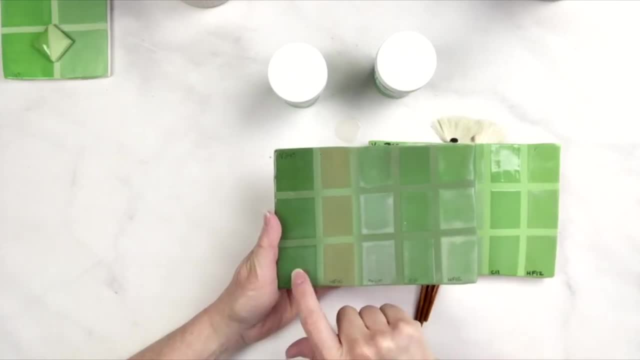 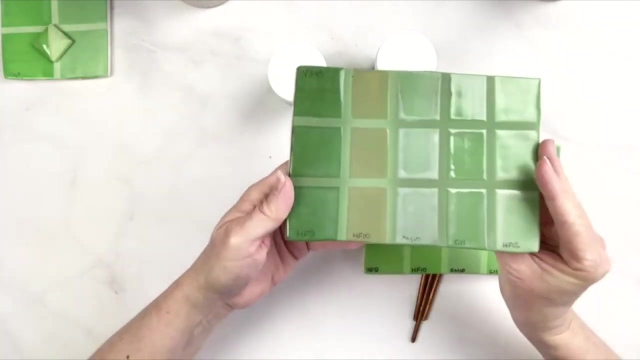 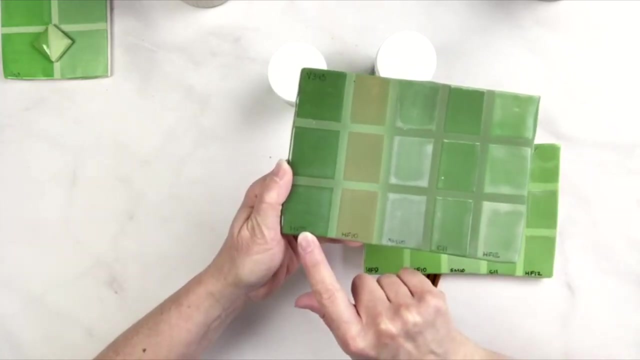 And you can see the difference between the Zinc Free and the Zinc changes that under glaze color rather substantially to a brown. Can you see that I'm trying to do this without getting too much reflection? It's more brown, Whereas with Zinc Free is more green. 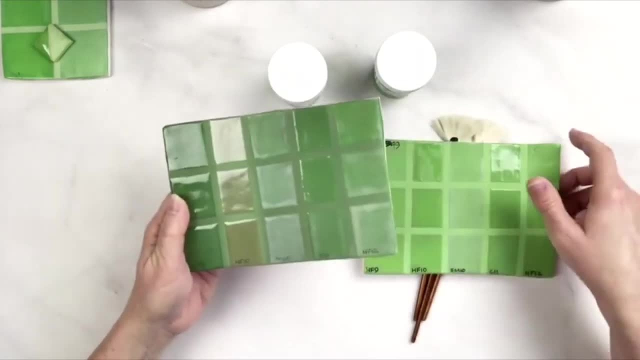 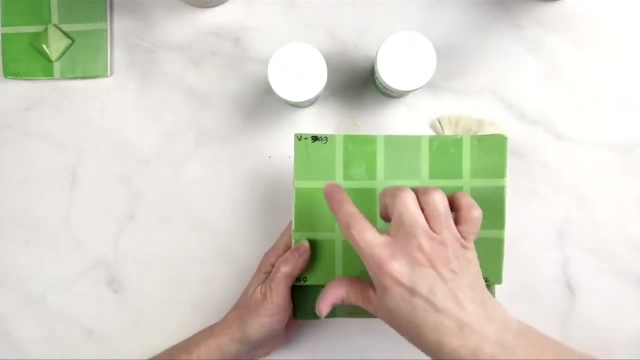 More true to color. You will also notice that it is a little bit darker. So there is a variation. And if you're wondering about the grid, this is: one coat, two coat, three coat of each of the clears. One coat, two coat, three coat. 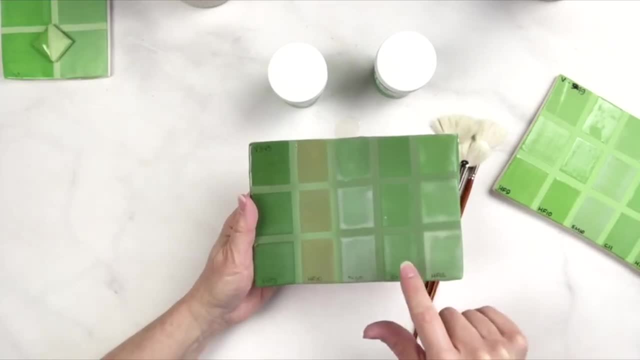 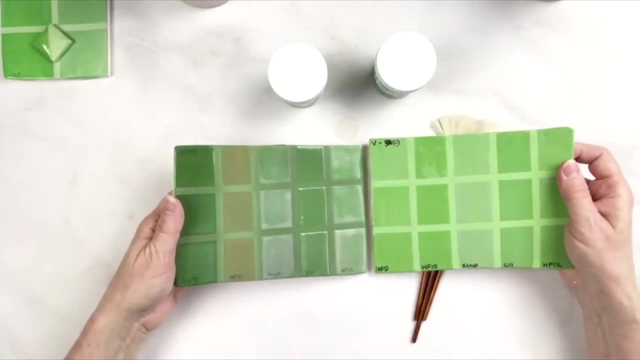 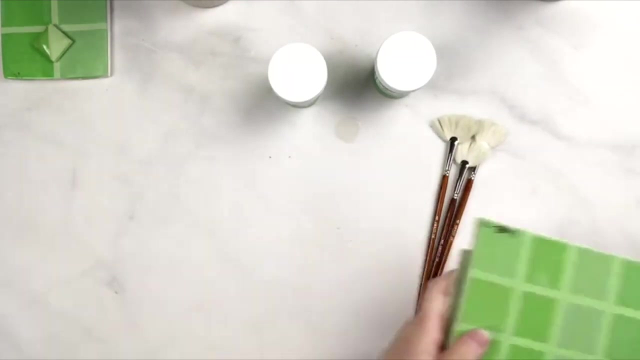 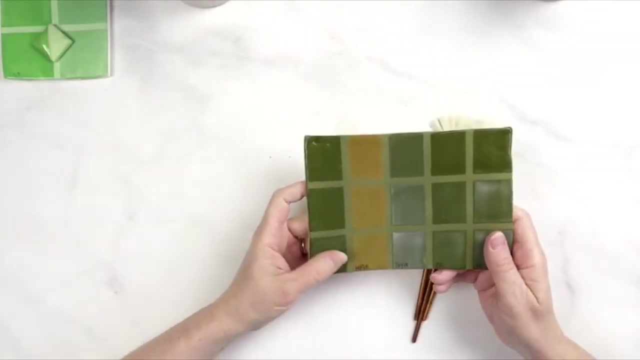 HF9, HF10, SM10, C11, Mixing Clear HF12.. So that was the purpose behind those new pink and green. I'm going to show you a more dramatic difference than Cactus and Light Green. We have Avocado Green Cone 5, HF9, HF10.. 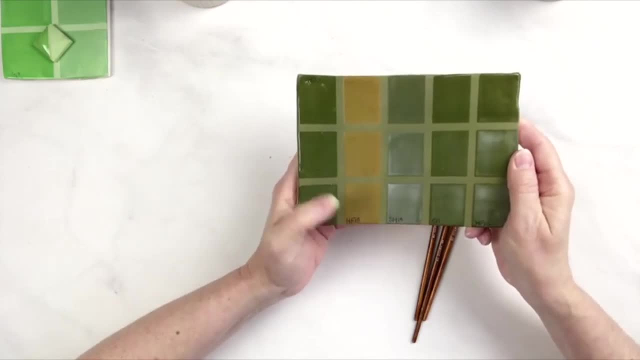 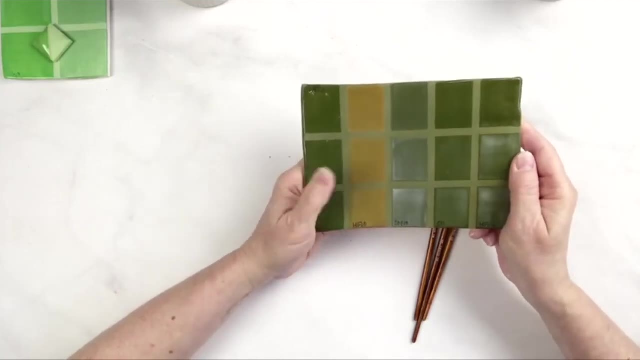 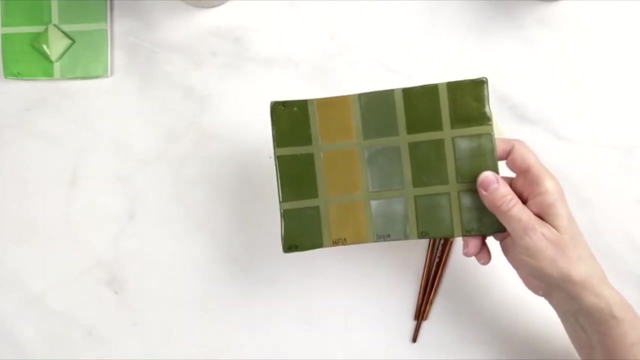 Can you see how much of a difference that makes? It is a very yellowy brown, Really a dramatic difference. Now, this is due to the kind of colorants that are in certain colors And interestingly, that same colorant is also in pinks. 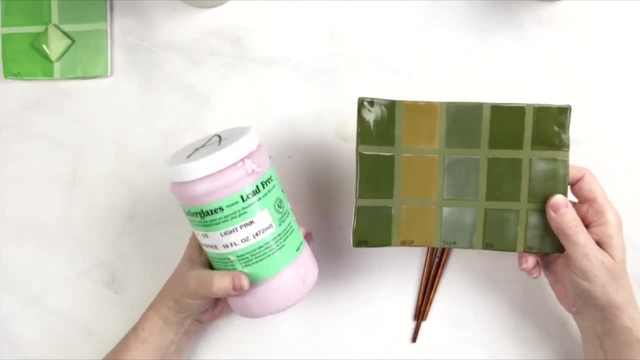 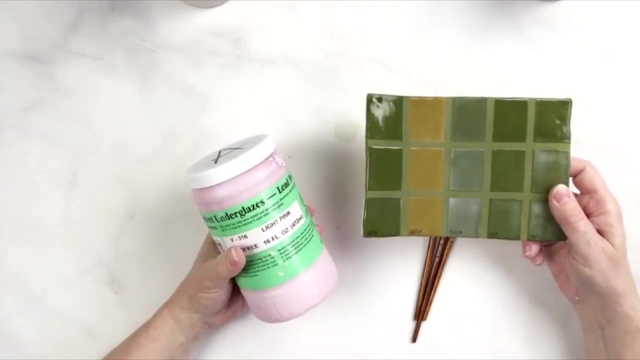 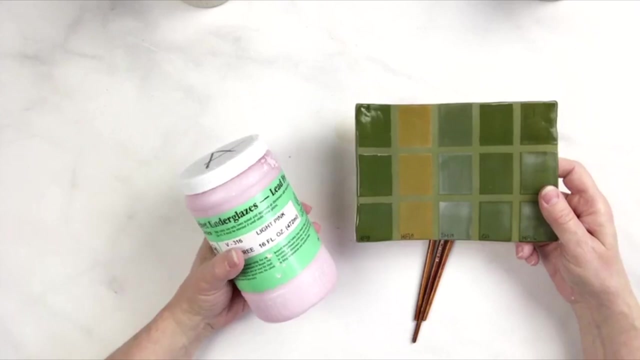 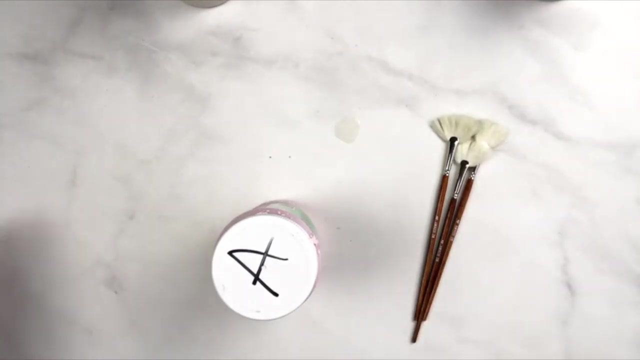 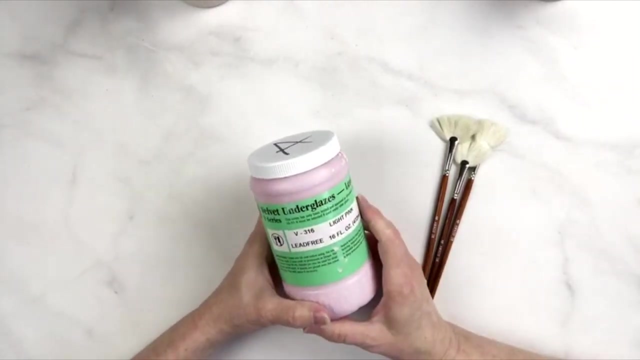 So if you are relatively new to glaze chemistry or you have not done a lot of mixing of glazes yourself, you may not realize that a lot of the colorants we use are the same, even though the colors themselves are dramatically different. So Chromium is the colorant in the older green underglazes and it will create a warmer tone with the presence of zinc. 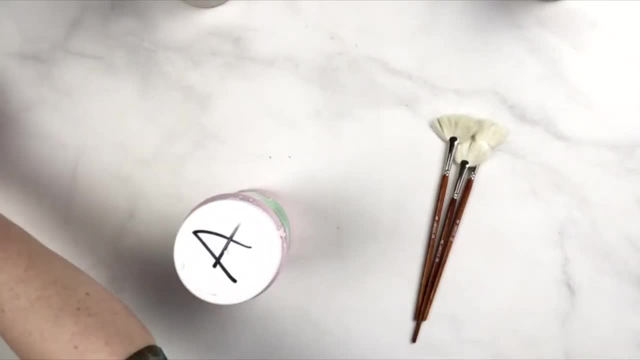 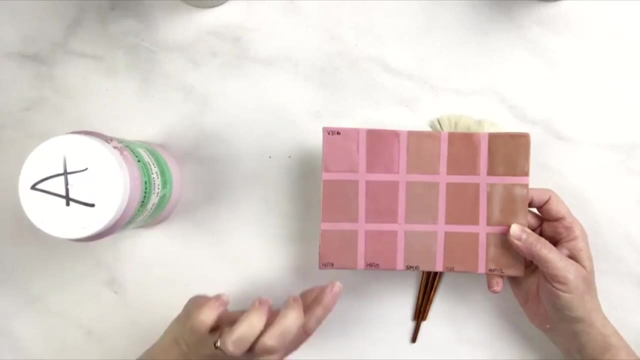 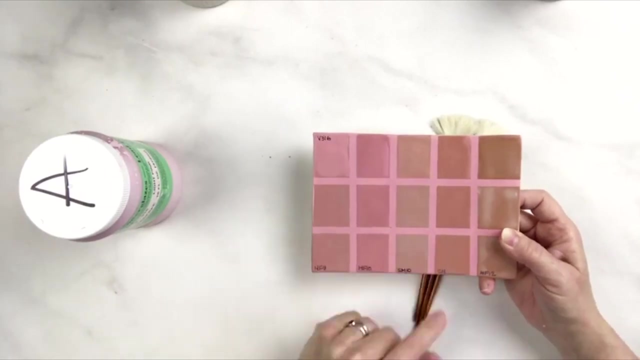 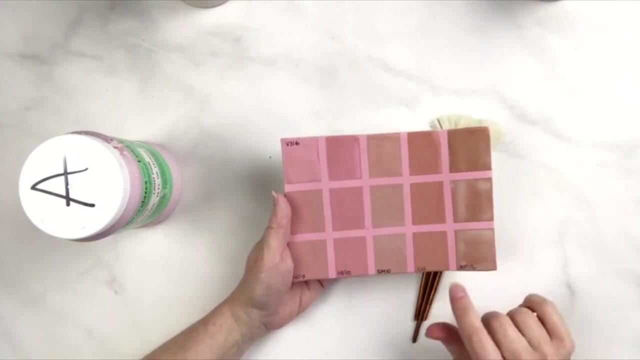 Now the funny thing is that that actually works for pink underglazes. So here is V316: Light Pink. HF9 is a little more brown. HF10 is a little more pink. HF10 actually looks pretty good. SM10 without zinc is a little bit brownish, as is the Mixing Clear and the HF12 has a very beige undertone. 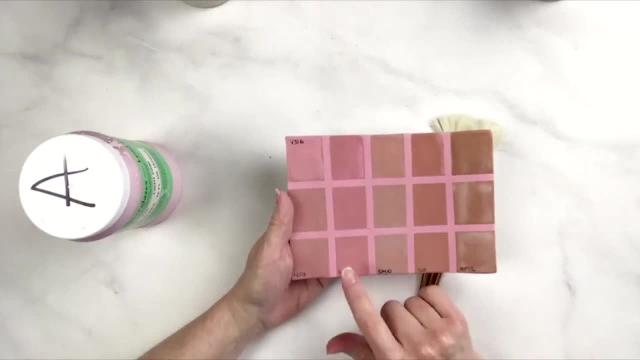 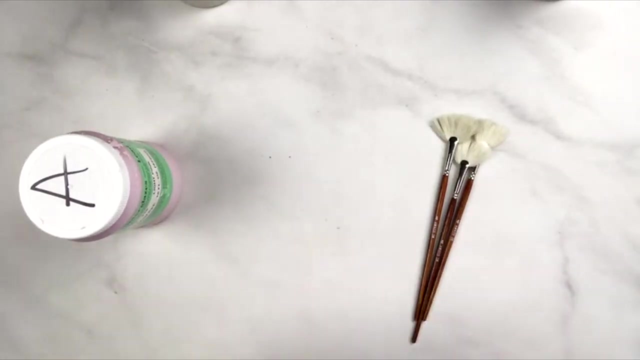 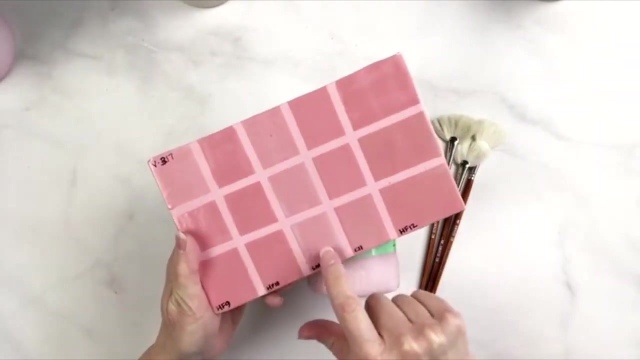 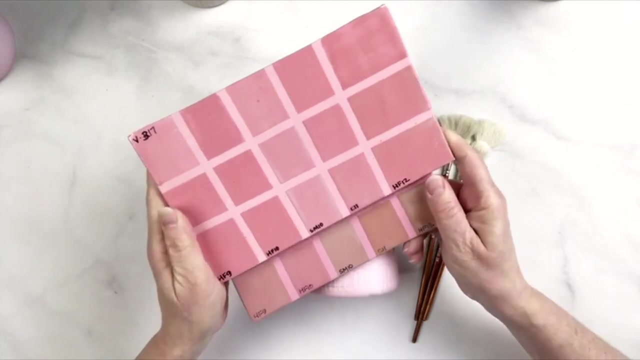 So what I used to say is pink likes zinc. So the pink actually did. the old Chromium pink did better with the presence of zinc than without. So We created V317 Coral and now, regardless whether you are using zinc or zinc free, you get the same bright pink all across the board. 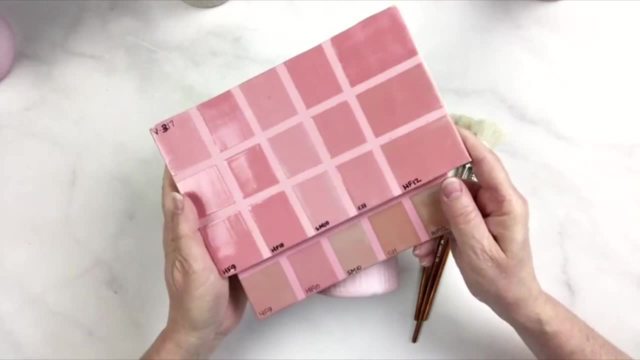 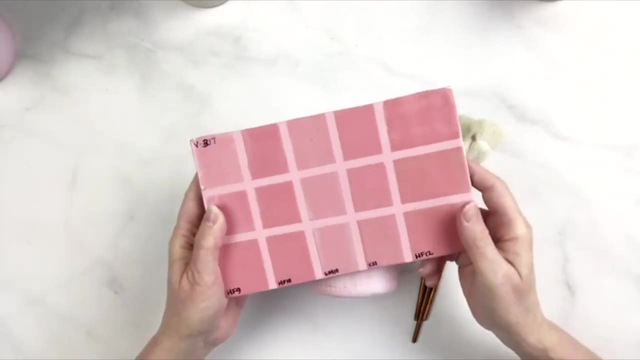 Isn't that nice. So that was the purpose. if you were wondering why we suddenly had two new pinks and two new greens when we already had pinks and greens, This would be why. So when we suggest a zinc free clear for underglazes, 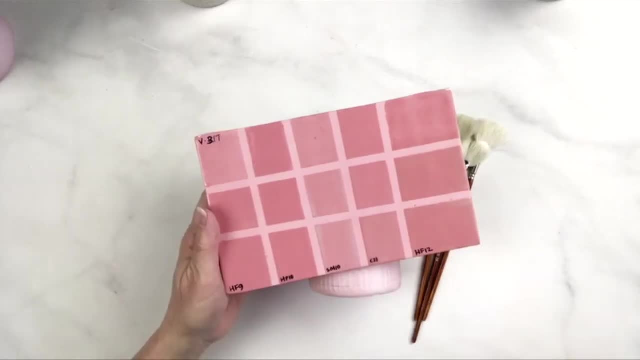 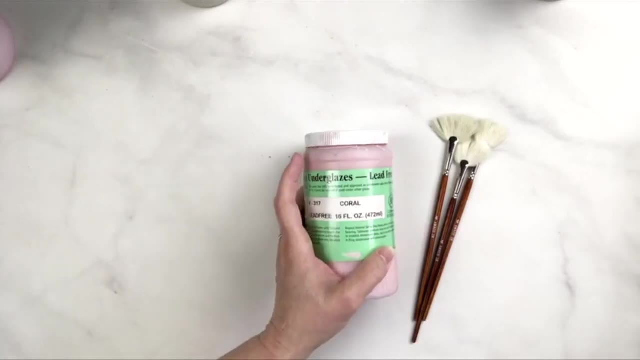 especially if you are using older formulations, it is to keep the colors as true as possible, Because certain colors will change. So The other question that I sometimes hear is about smudging, Smudging and dragging. So I've had some people who suggest 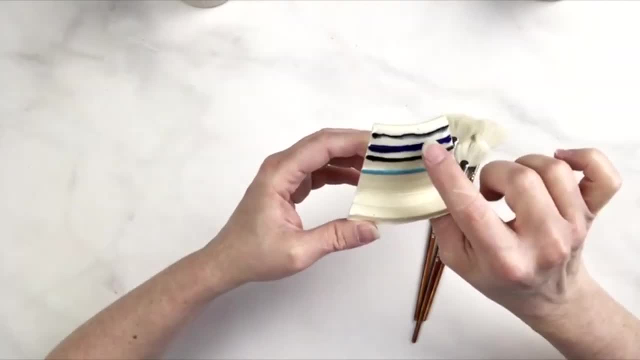 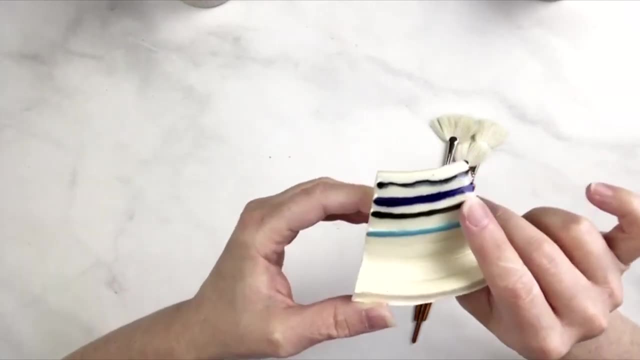 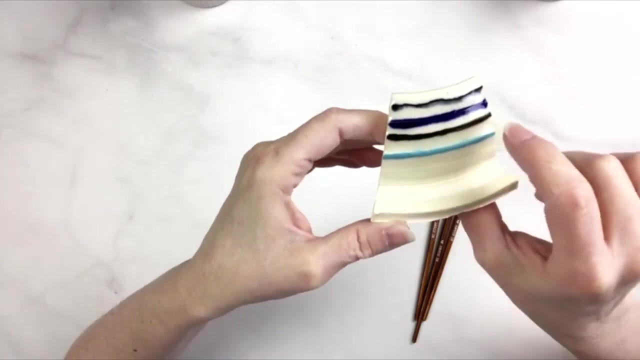 and you can see here in this tile. you see how that top line is like dragging down- I don't know how visible that is. The next line isn't really doing that, The line below is not doing it and the fourth line is not doing it at all. 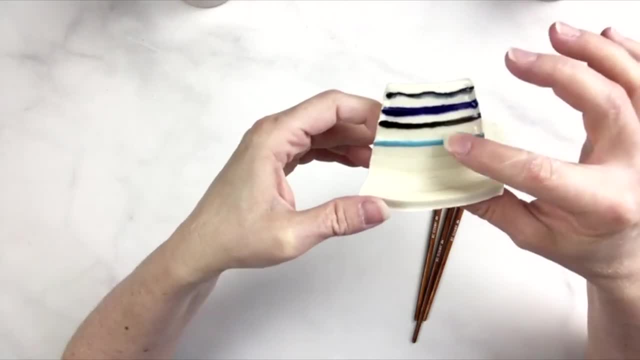 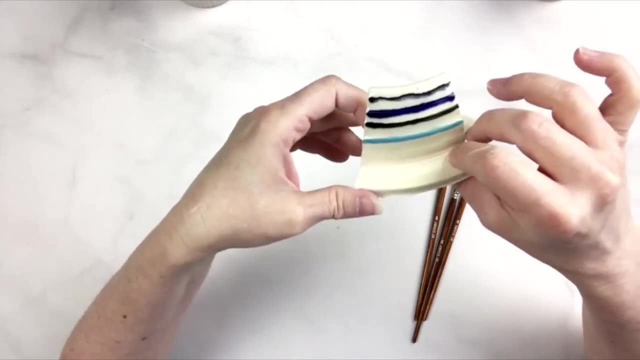 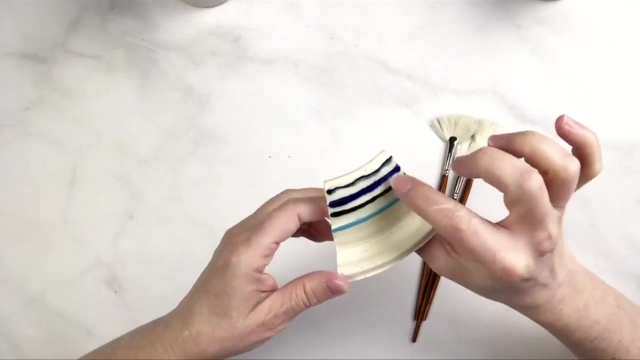 So some underglazes will drag with some glazes. It depends on the glaze and it depends on the underglaze. So in this case this is HF9 Zinc Free Clear over four different underglazes. The top is V370 Velour Black. 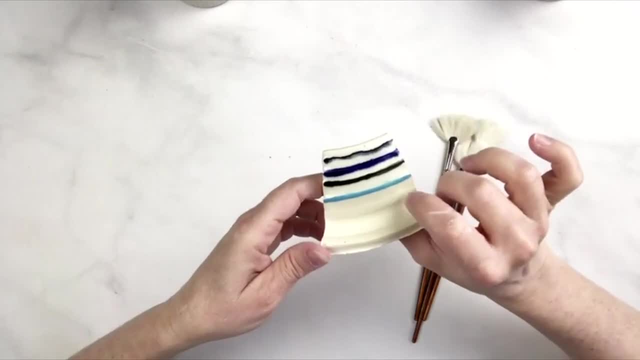 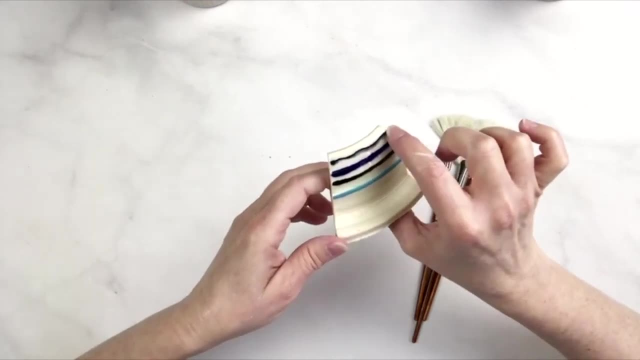 which we use for a great many things, and it does not flux even as high as Cone 10.. But the glaze did drag it a little bit because it was a very thick line. The second line was: let me check my notes. 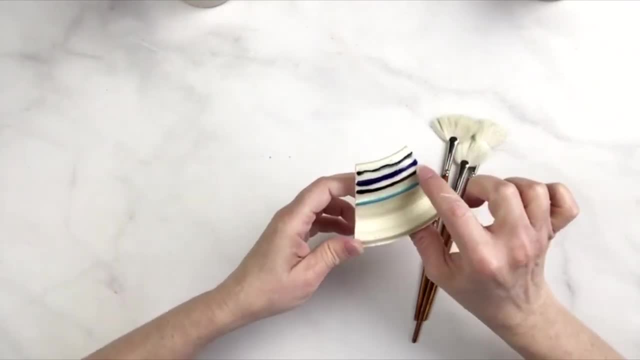 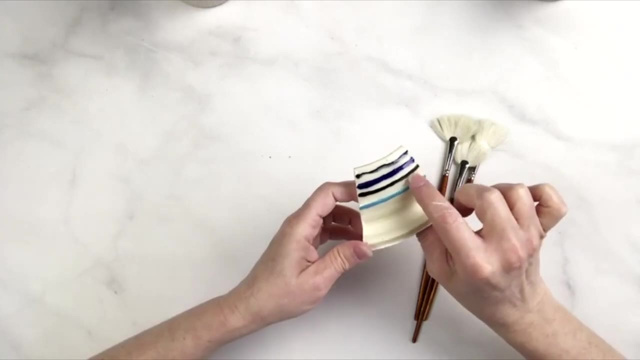 V336, Royal Blue, and it looks a little bit hazy at the bottom, but it's not really dragging. The next one is Jet Black V361, and it didn't drag, which is interesting because it will flux. And the fourth line is an LUG. 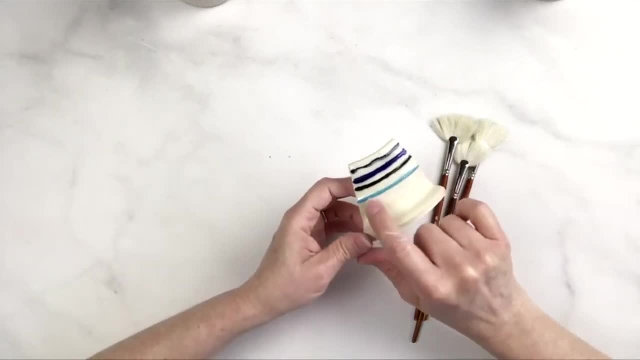 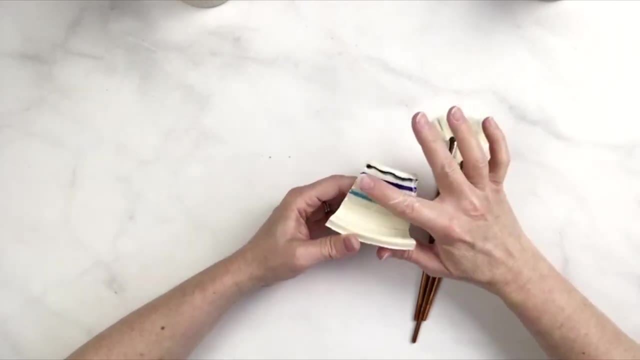 LUG 20, and this one absolutely fluxes. It's almost a glaze at Cone 6, which this was fired to, And yet it didn't move at all, because what's happening is the glaze is dragging the colorants. 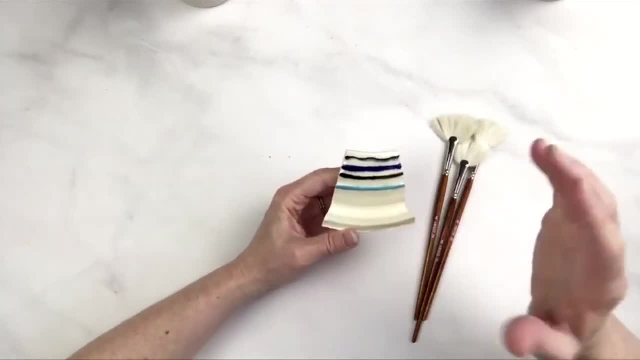 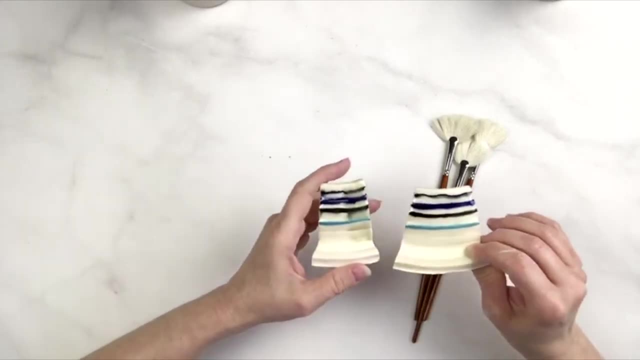 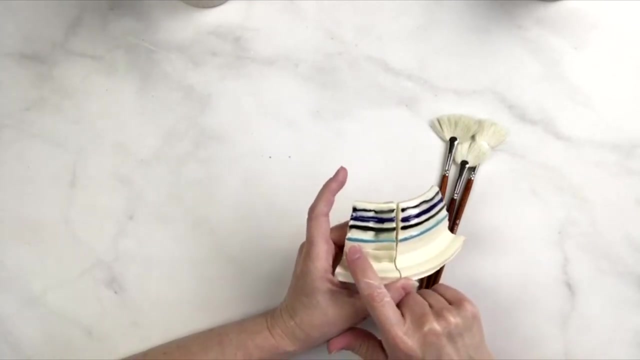 And especially glazes that are very high in colorants, and a glaze that moves a lot will drag more. So I did a few different things, same lines, but you can see how different glazes. HF 12, this is LG 10,. 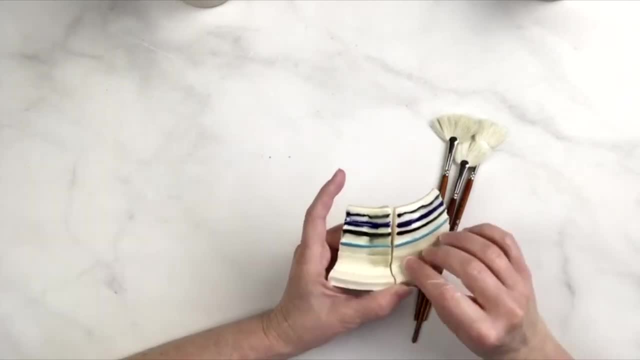 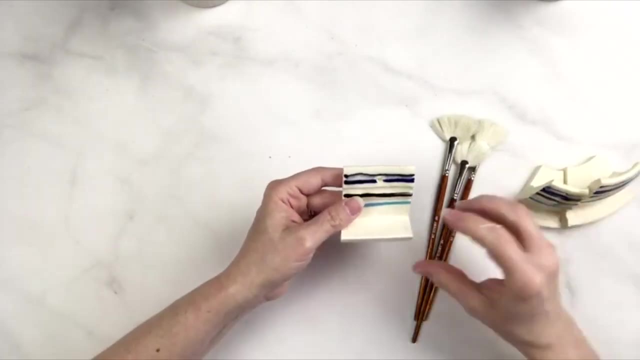 a low fire clear glaze fired to Cone 6 just to see what it would do, And it moved the underglazes a little bit, but not a lot. And this is HF 10, and you can see it kind of bubbled more. 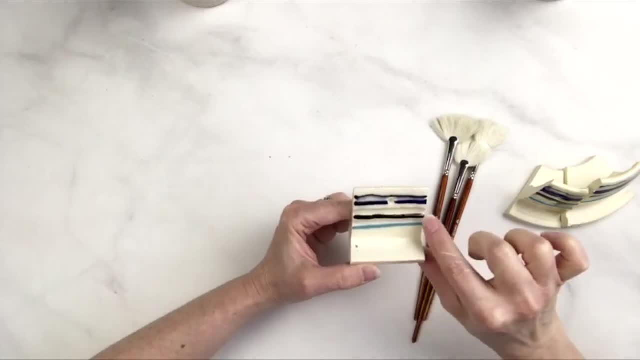 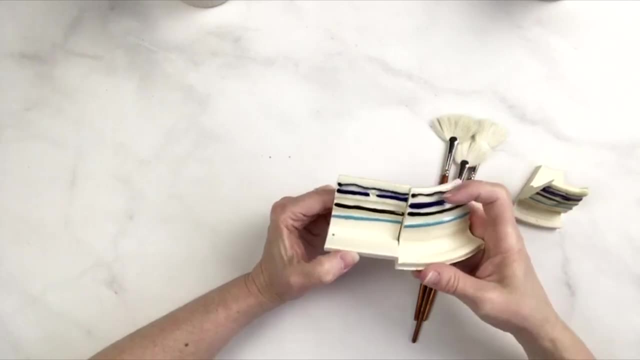 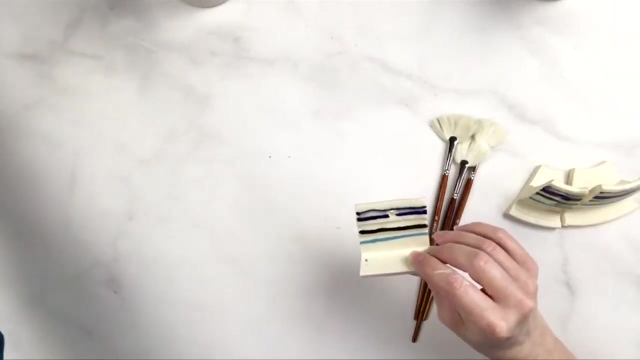 and it didn't drag at all on the Jet Black. It did drag a tiny bit on the Velour Black, but you still have a better line, a crisper line, with the HF 9 Zinc Free. And then, just to see, I used an extremely runny glaze. 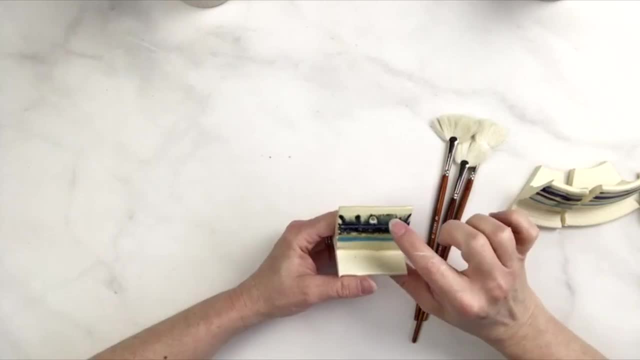 and this is not an Amaco glaze, but it is a very runny glaze- and it dragged the Velour Black to the point where it almost isn't even on the piece anymore, as well as the Jet Black and the Royal Blue, 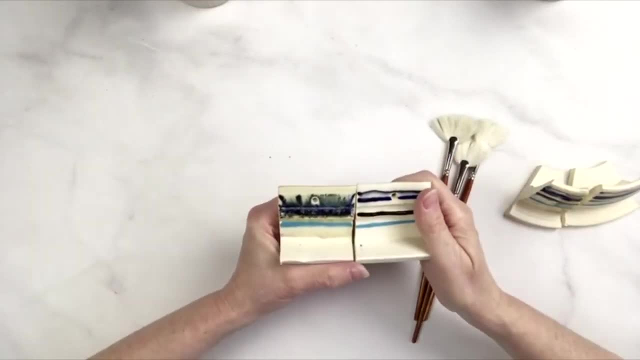 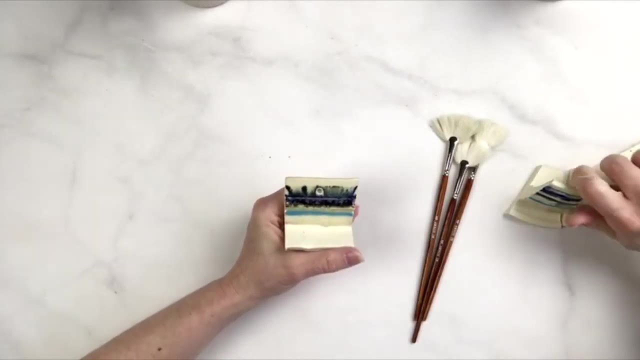 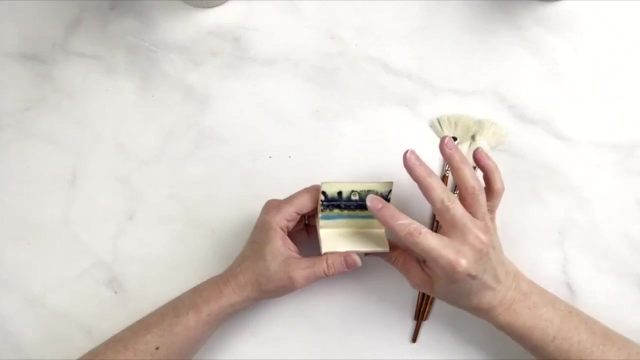 were just completely dragged, So you can see how those were lines. and then they're not lines anymore, They're just all over the place. So dragging is partly a process that happens because of the movement of the glaze rather than the underglaze itself. 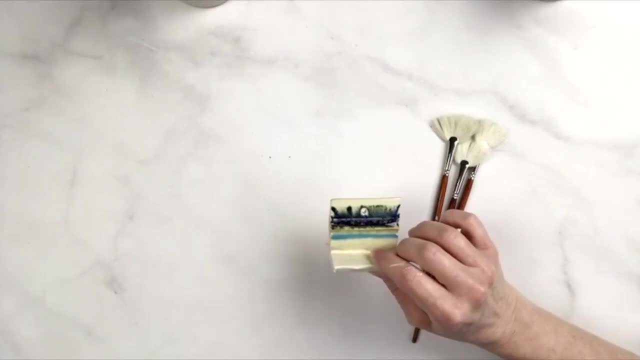 Sometimes people are worried that it has to do with applying their clear glaze, that they need to worry about smudging. It's not always smudging, Sometimes it's dragging. So if you hear me talk about something being dragged, that's a little different. 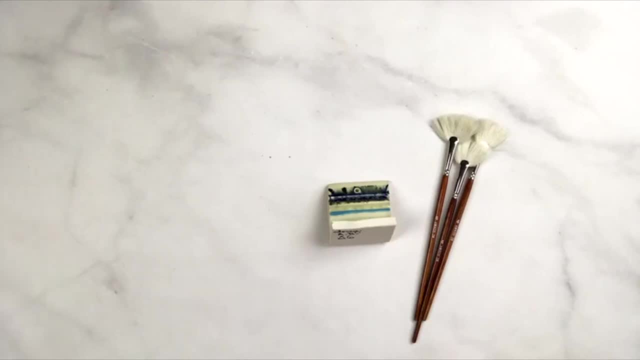 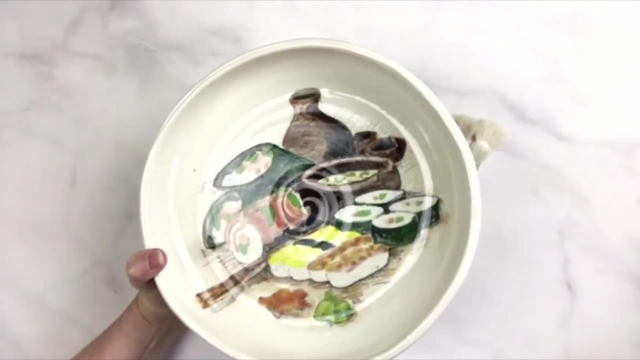 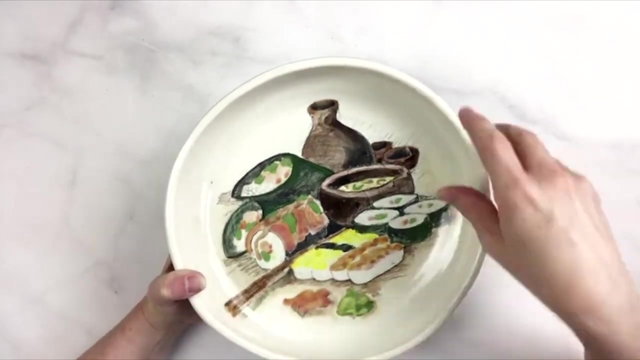 Now, a couple of weeks ago, I did a demo with the smugs and I did not bisque fire it before I applied the clear glaze. I just applied the clear glaze right on top and fired it to Cone 6,. 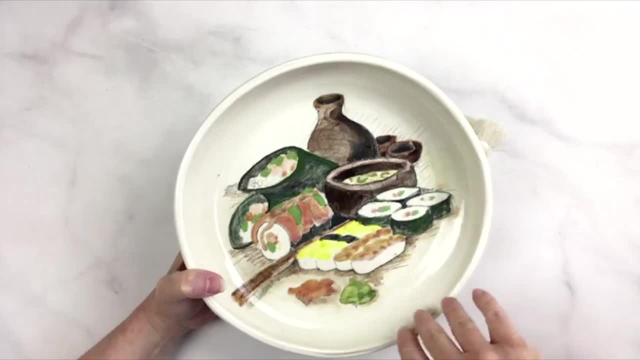 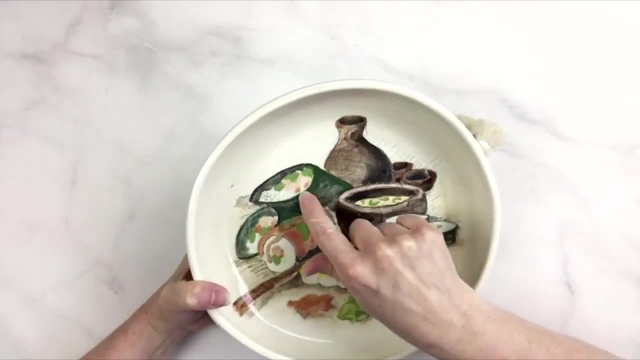 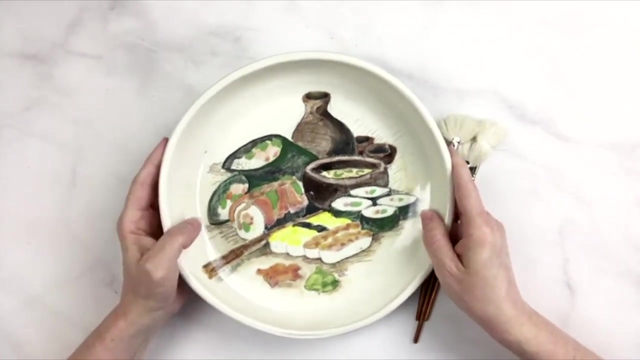 and you can see that the colors are a little different. Some of them are a little bit washed out. I lost some of my detail around my rice. Some of the colors are still very, very opaque and some are more transparent. Now you'll notice that I don't have smudging. 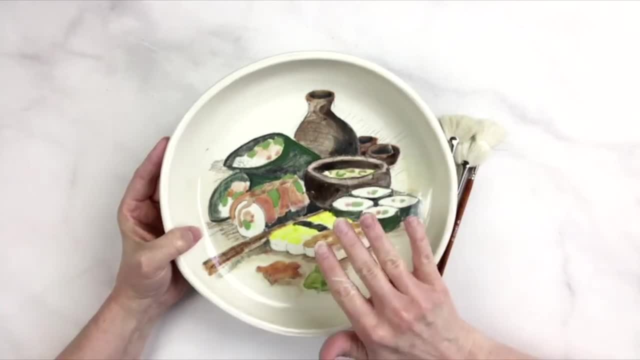 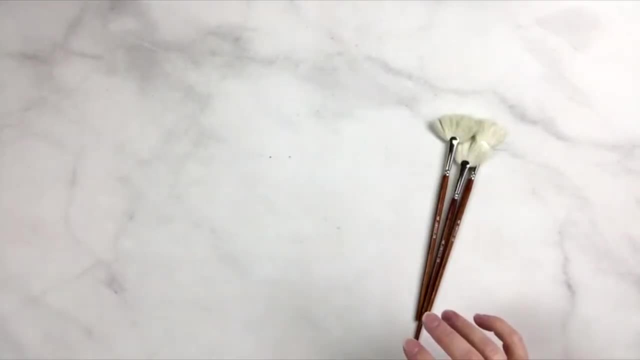 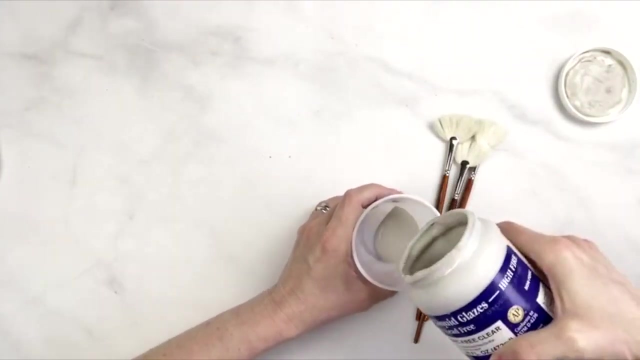 The colors are softer but they still look the same. They didn't move And what I did to apply that first coat of glaze was: I took a little bit of my glaze and you can do it out of the jar, but I find it easier to do it in a small container instead. 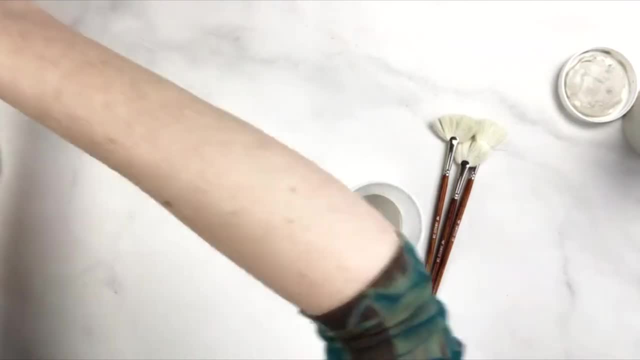 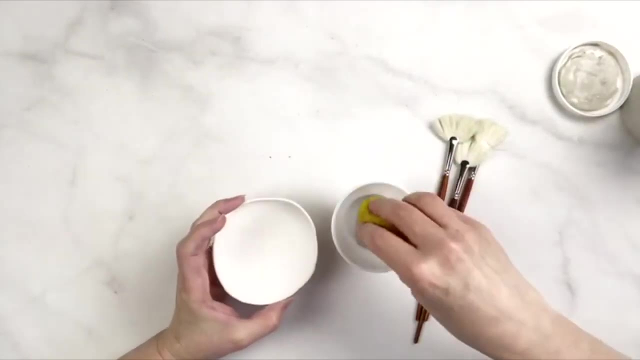 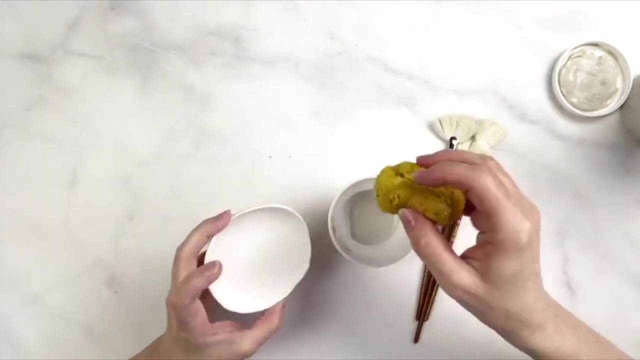 And with a clean, damp sponge- and I don't have something that has underglaze on it already, which would make it easier to see what I'm doing- but I take a sponge- clean sponge- and gently dab the glaze on. 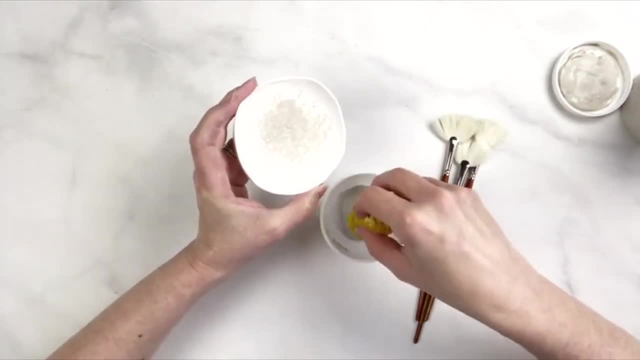 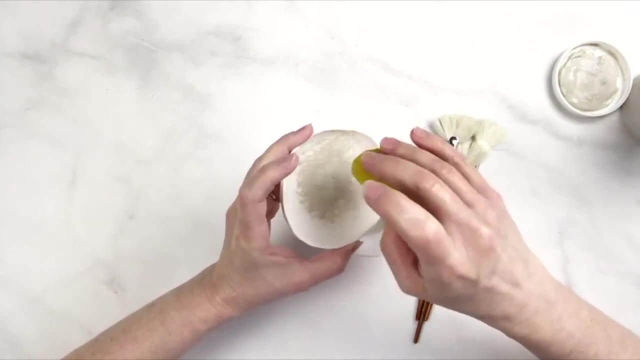 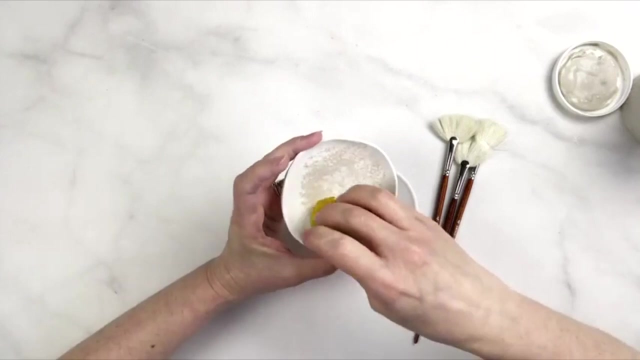 for the first coat. Now, once this is dry, you can go back and you can brush right over. But if you're worried about smudging and smearing your underglaze, you can always apply it as a sponge coat first. So just sponge it on gently. 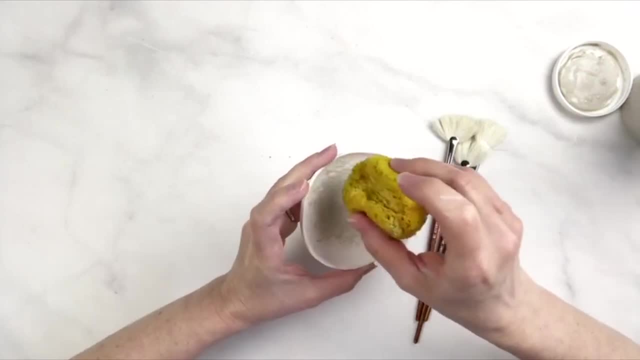 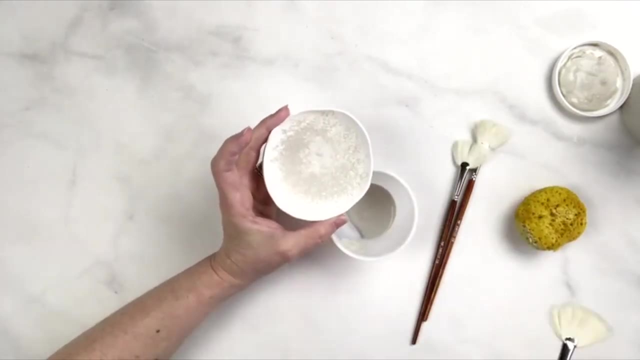 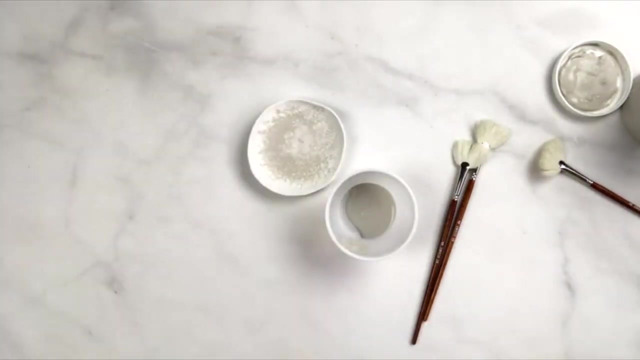 Do the whole surface And then, once that's dry, just take a brush, brush on normally for your second and third coats. So I do always recommend that people make their own test tiles to see how- not only how- the underglazes will look. 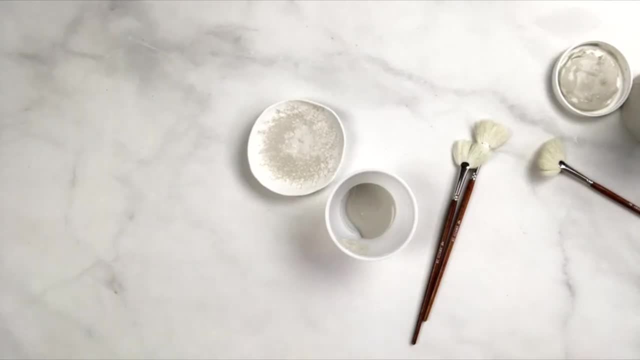 but also how they look, the way that you apply them. So generally, underglazes need to be applied three coats And then, when you're done, to be opaque. So if you're using the velvet underglazes, we do recommend three coats.